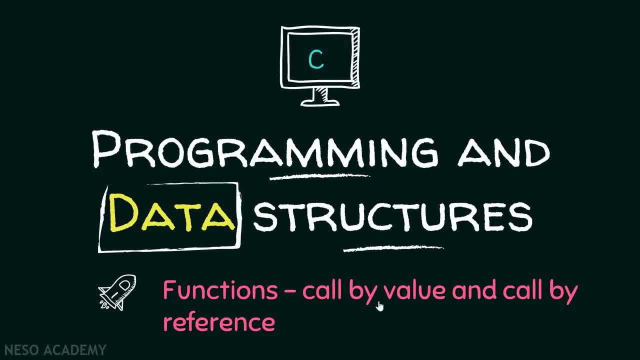 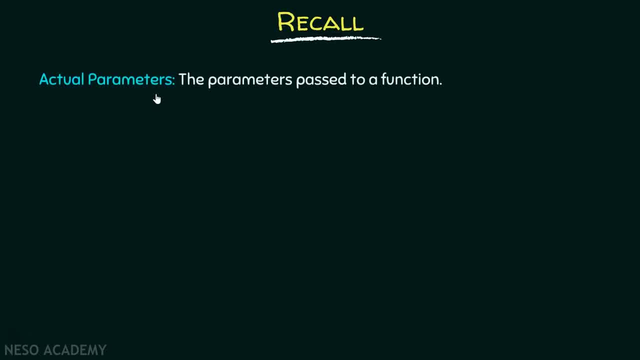 In this presentation we will talk about functions called by value and called by reference. So let's get started. Recall that actual parameters are the parameters passed to a function and formal parameters are the parameters received by a function, Like, for example: here is the calling procedure for a function: add right. 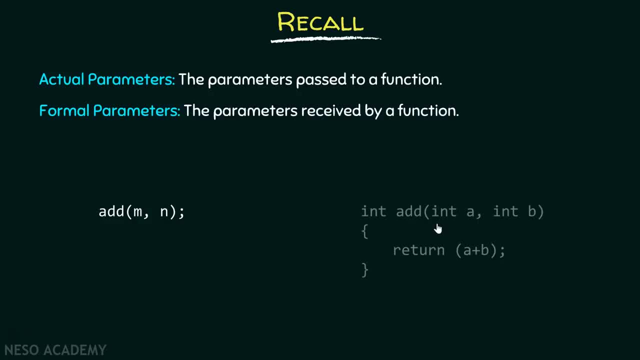 This is the way you call a function, right, And here is the definition of this function. add: When you are calling this function with m and n as the parameters, then the value of m will get passed to the variable a and value of n will get passed to variable b. 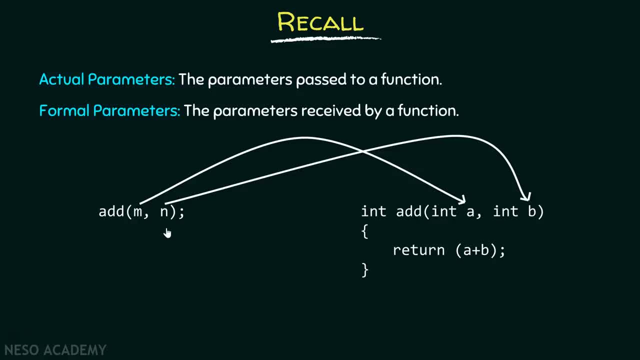 This is how it works, right? So these parameters are called as actual parameters because these are the parameters passed to a function, and these are called as formal parameters because these are the parameters received by a function, right, As they are receiving the values. therefore, they are called as formal parameters. 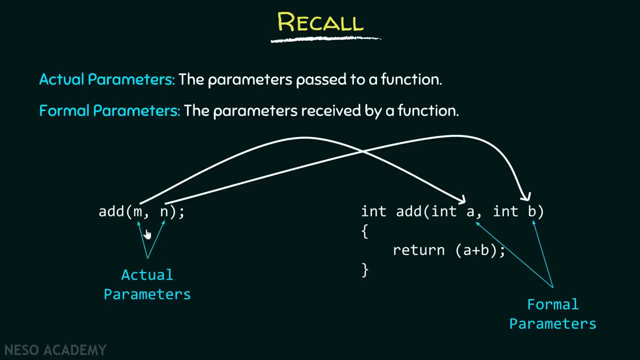 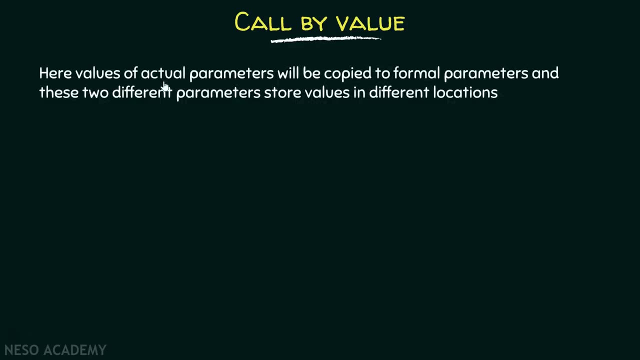 and they are sending the values. therefore, they are called as actual parameters. Okay, Now let's try to understand what is called by value and what is called by reference. Let's first try to understand what is called by value. Here, values of actual parameters will be copied to formal parameters. 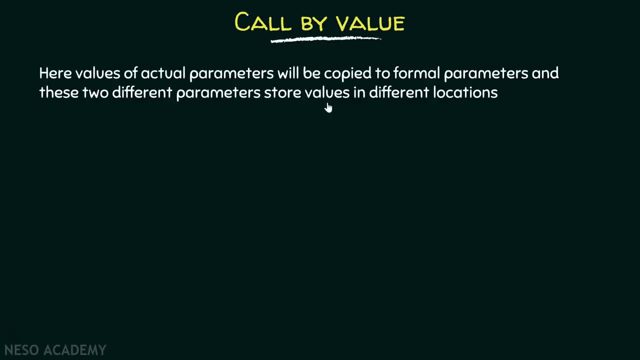 and these two different parameters store values in different locations. We have these two variables x and y. Let me declare these variables over here: Variable x and variable y. Variable x contains value ten and variable y contains value twenty. right, What we are exactly doing in this calling procedure? 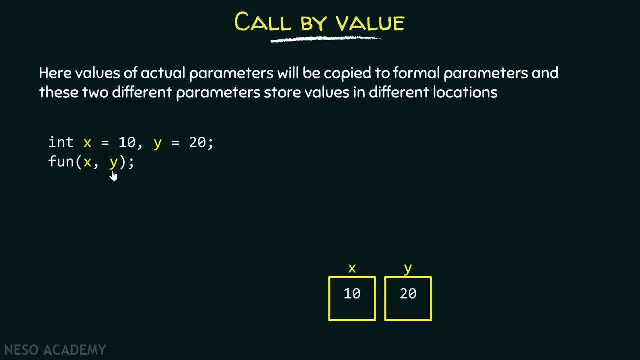 we are passing the values of x and y to the function definition which is available over here. These values ten and twenty will get passed to these variables x and y. Let me declare these variables over here: x variable and y variable. These variables now contain value ten and twenty. right. 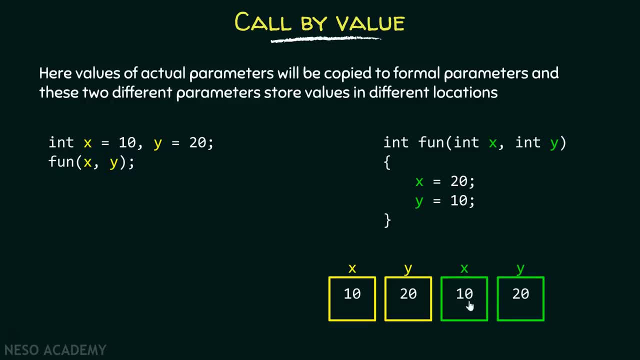 Now, inside this function, we are changing the value of x to twenty. That is what we are doing here. And we are changing the value of y to ten. That is what we are doing here. So variable x will now contain value twenty. 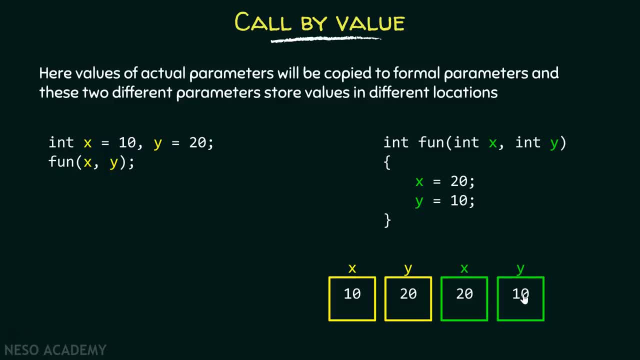 and variable y will contain value ten. Now please note down that these variables are local to this function. When this function procedure finishes, we get back to this calling procedure, Then these variables will get destroyed, right, And whatever the changes you made in these variables. 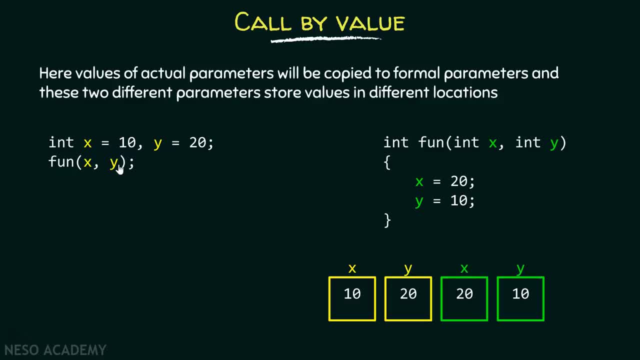 will not get reflected back to these variables. So if we try to print the values of x and y, then the output is x equals to ten and y equals to twenty, which are the original values. This is what we need to understand about the call-by-value. 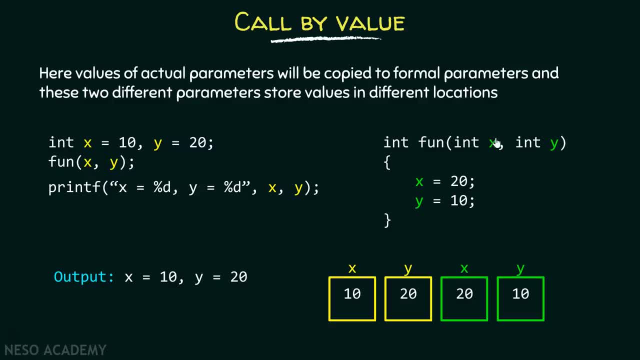 In call-by-value procedure, you are simply passing the values to the variables and not the variables itself. So whatever the changes you made to these variables will not get reflected back to these variables. This is called call-by-value. Now let's try to understand what is call-by-reference. 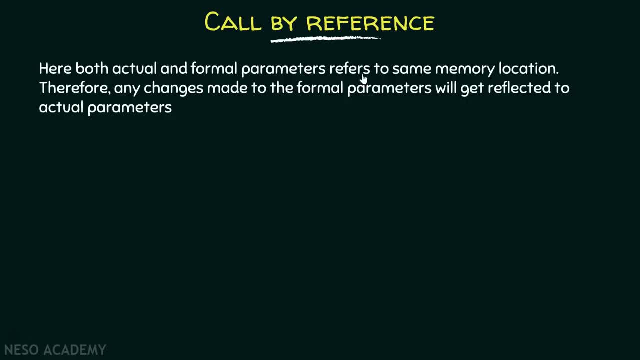 Here, both actual and formal parameters refers to same memory location. Please note down this point. Therefore, any changes made to the formal parameters will get reflected to actual parameters. Whatever, the changes you made to the formal parameters will get reflected to actual parameters. 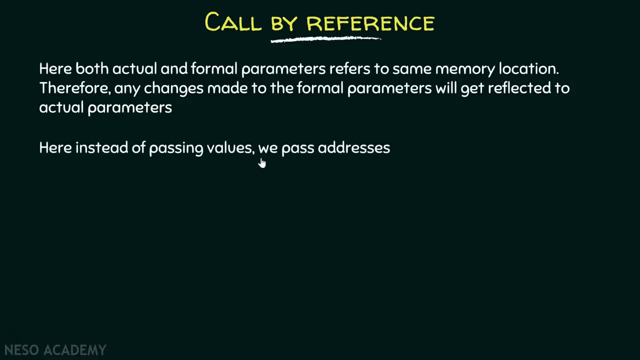 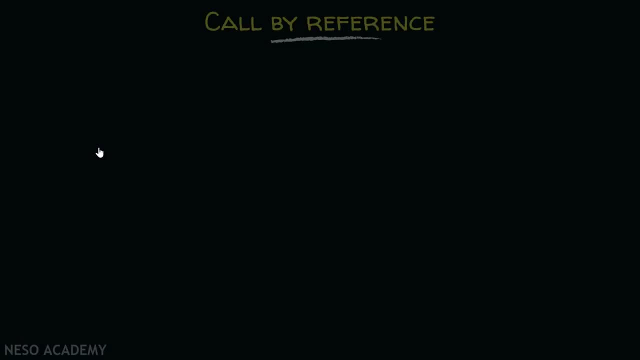 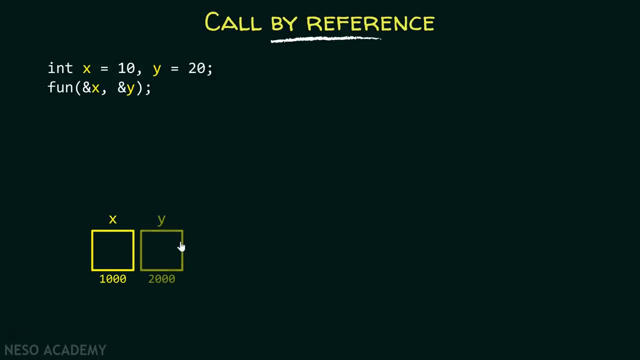 Also here, instead of passing values, we pass addresses. We are not passing the values, we are passing the addresses. Like for example here: we have two variables, x and y. Let me declare them over here: Variable x and variable y. 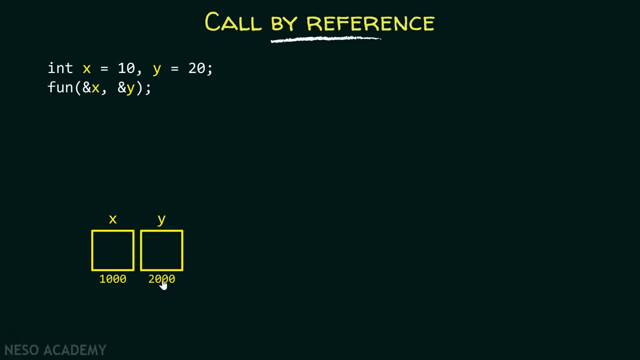 And they have addresses one thousand and two thousand respectively. Now the value of x is ten and value of y is twenty. So in this calling procedure you can notice the difference. Here, instead of writing x and y directly, we are also mentioning these ampersand operators. 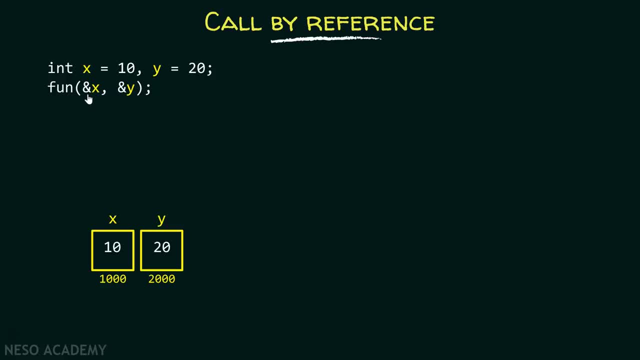 Which are also called as address of operators. That means we are simply passing the addresses of these variables Instead of passing the values. Here ampersand of x means address of x and ampersand of y means address of y. In the definition of the function, 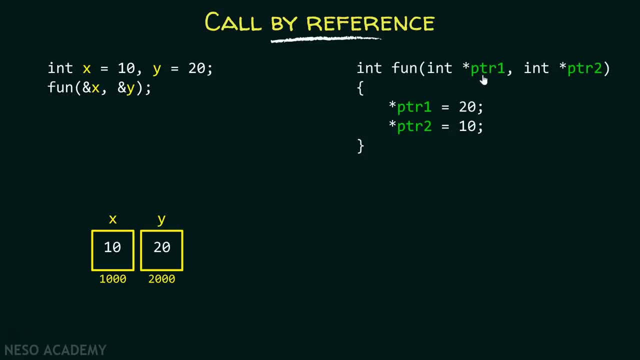 address of x and y is received instead of values. Okay Now, as addresses are received by this function, therefore some special kind of variable is required to store them, As if we simply declare a variable over here in the parameters list, then they are not capable enough to hold the addresses. 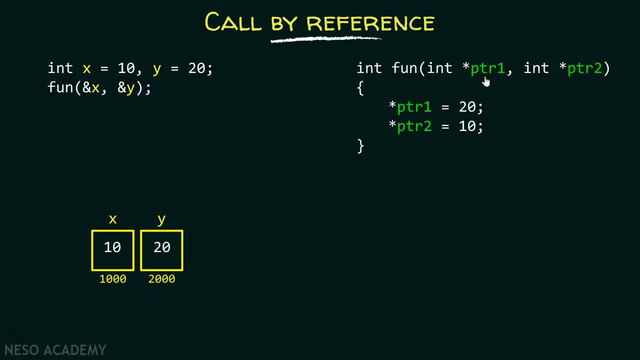 Therefore, we require special variables, which are also called as pointers. Pointers are those variables which can store addresses of some other variables. This is the way you declare a pointer. We will talk about pointers later in greater details, But right now it is important for us to know. 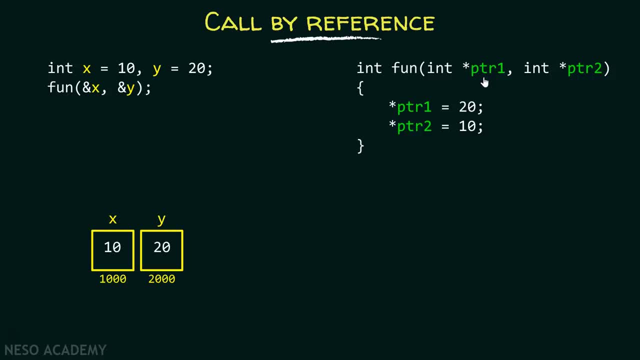 that pointers are those variables which can store addresses. Let me declare these pointers over here. This is ptr1 and here is the ptr2.. ptr1 stores the address of variable x, which is 1000.. Therefore, 1000 will get stored. 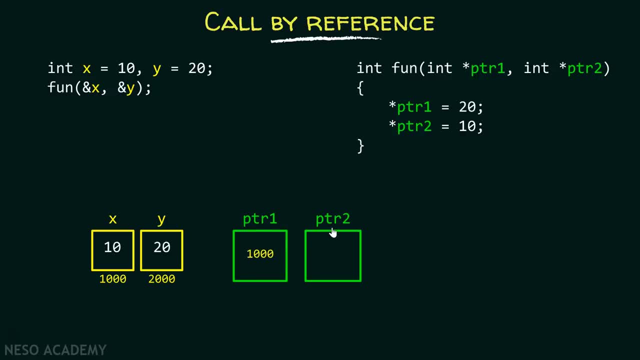 inside this pointer, ptr2.. And ptr2 will store the address of variable y, which is 2000.. Now inside this function, we have two statements: star ptr1 equals to 20, star ptr2 equals to 10.. Now here is one important point. 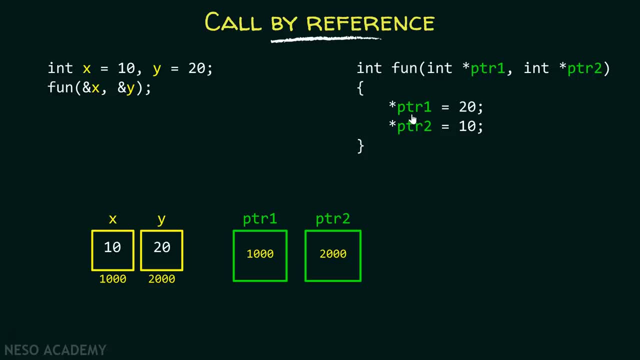 we need to understand. Whenever we simply write a variable- suppose x- then this simply means that we are accessing the content of that variable. Now, if we write simply ptr1, that means we are accessing the content of ptr1.. The content of ptr1 is the address. 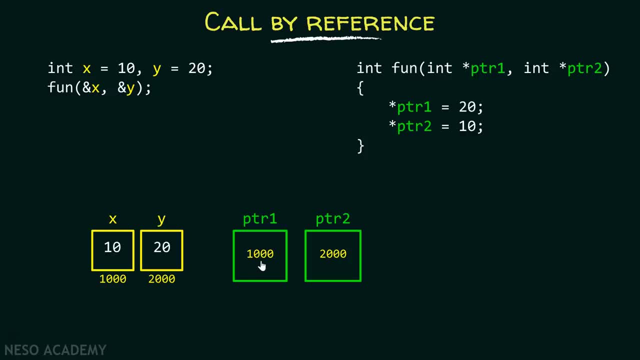 of the variable x right, which is 1000.. If we write star in front of ptr1, this simply means that x is the value of that particular address. Okay, This particular operator is called as dereference operator, which is just opposite to. 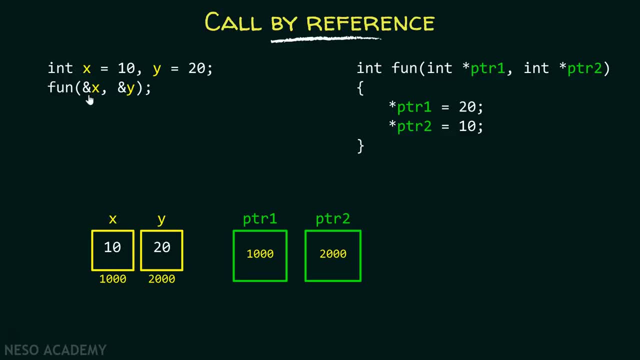 this operator ampersand. It is also called as reference operator. So what does it really mean? When we simply write ptr1,, we are accessing the content of ptr1, which is 1000.. Therefore, ptr1 will get replaced. 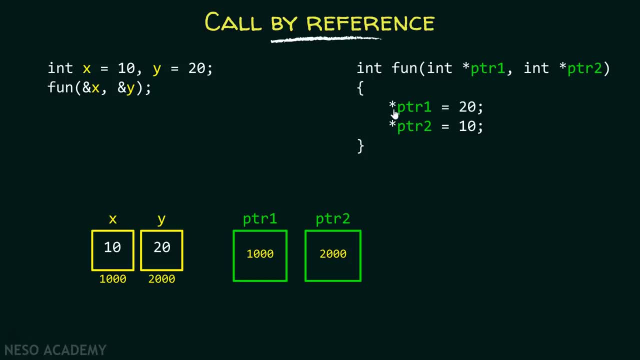 by 1000, right Now. when we write star in front of 1000,, that means we are trying to access the content of this particular address: 1000.. This means we are mapping 1000, right, And this simply means we are trying. 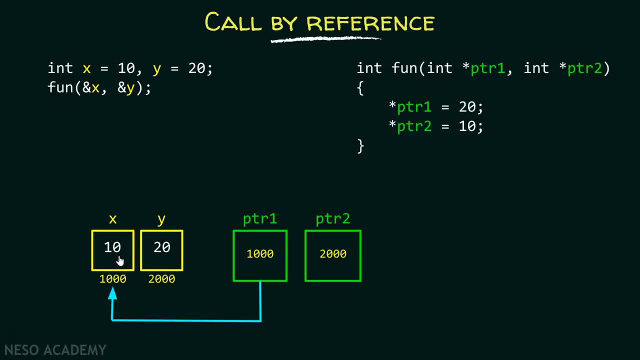 to access the content of variable x, which is 10.. Now here I am assigning 20,. that means we are changing this value to 20, right? Similarly, when we are writing ptr2, we are trying to access its content, which is 2000..